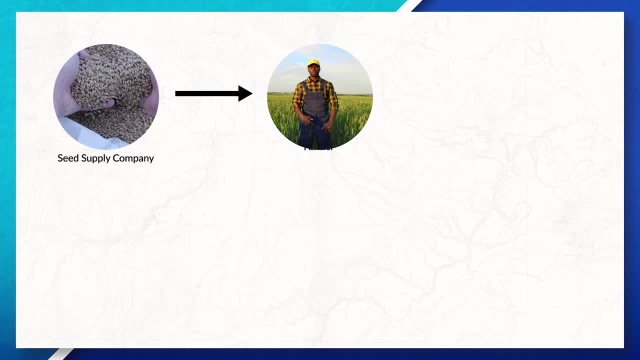 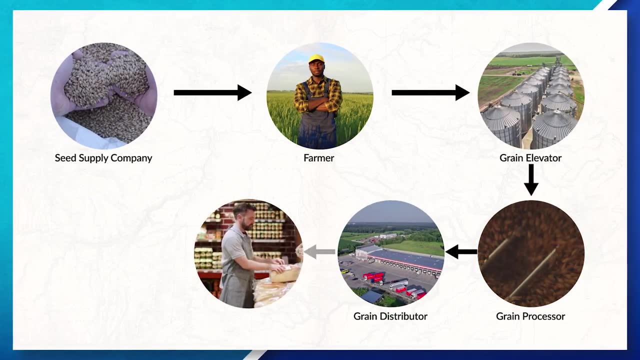 A commodity chain is a commodity chain that is built on a large scale. A commodity chain is a process used by companies to gather resources and transform them into a good and then distribute them to the consumers for sale. These chains encompass the entire production process, from the idea, the creation of the good, the design, production, the distribution and eventual sales. 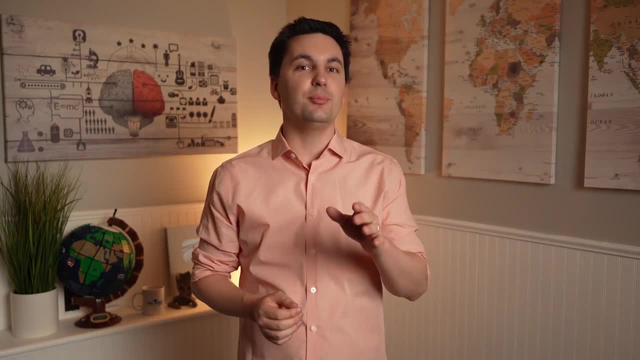 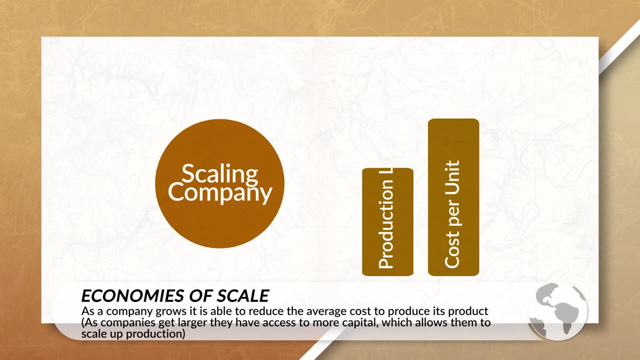 Now I also mentioned a concept you might not be familiar with, and that is economies of scale. This is when a company can reduce its average cost of production due to increased production levels. Essentially, as companies get larger, they can purchase better machines, systems and more. And they have more access to capital, which allows them to scale up, producing more of a product at a cheaper rate. Companies that have economies of scale are able to produce more at a cheaper rate, which gives them an advantage in the market. In agriculture, we can see, this is just one of the reasons why family farms struggle to compete with large corporate farms. 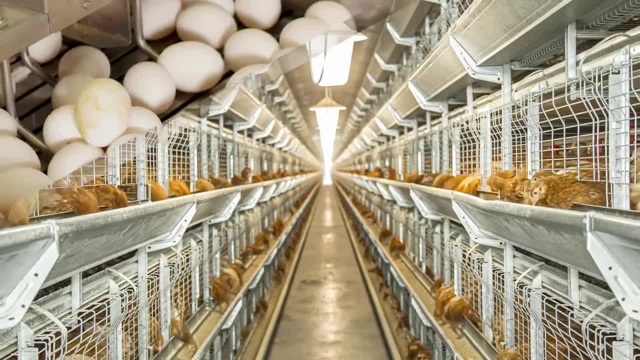 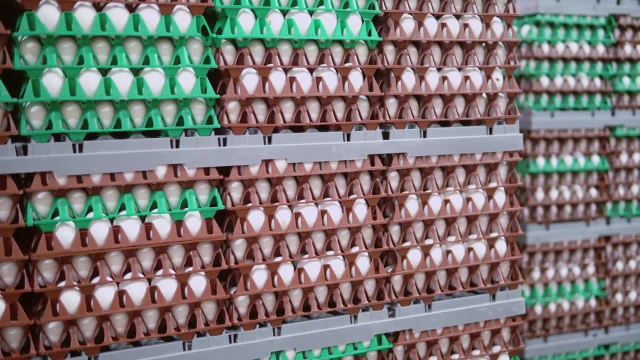 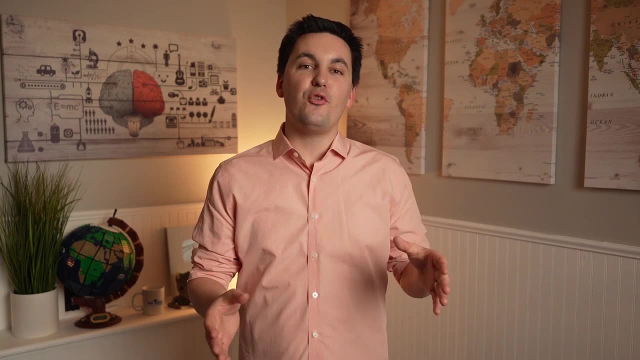 Large agribusinesses have achieved economies of scale. These companies have access to advanced machinery that can quickly produce lots of food, which lowers the average cost of production. Over time, we've started to see many family farms be purchased by larger farms to consolidate the farms under one business. 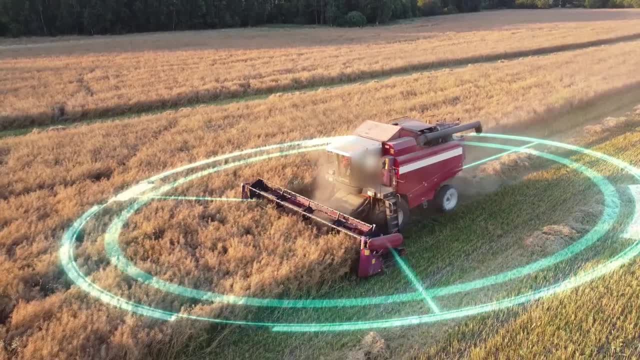 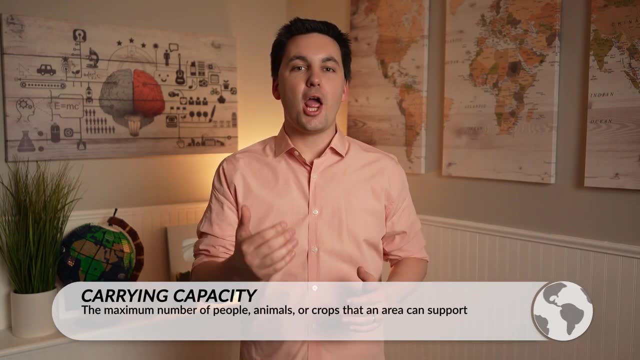 Today, we can see that industrial farming has continued to move towards automation and mass production, reducing the need for human labor in agriculture, All of which is changing not only our carrying capacity but our agricultural and physiological density as well, Concepts we last talked about in our Unit 2, Topic 1, video. 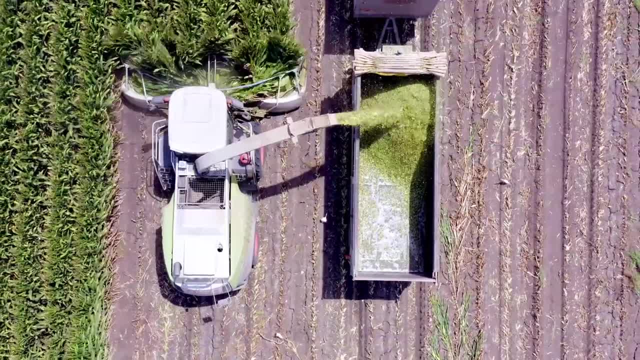 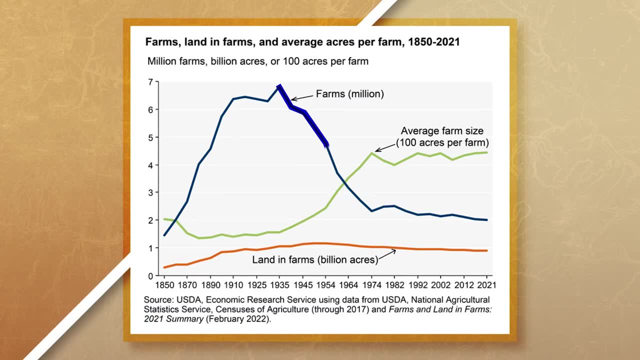 As industrial farming grows, so does the average size of a farm, All of which we can see here. when looking at data from the US Department of Agriculture, Notice how, over time, the amount of farms in the United States has decreased. 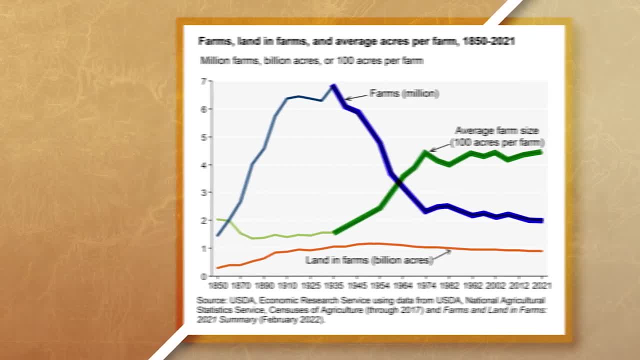 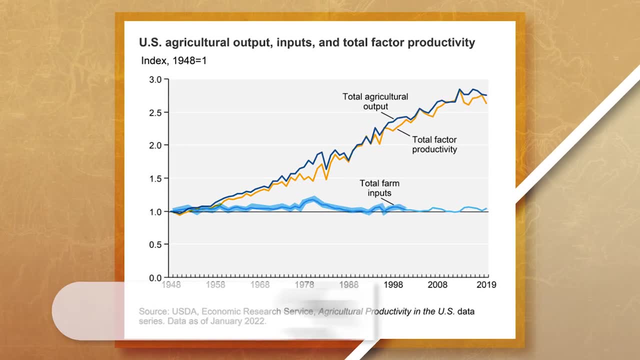 while at the same time, the average farm size has increased. We can take this further and look at agricultural production in the United States as well, where we can see total agricultural inputs have remained low. over the years, However, total agricultural output has significantly risen. 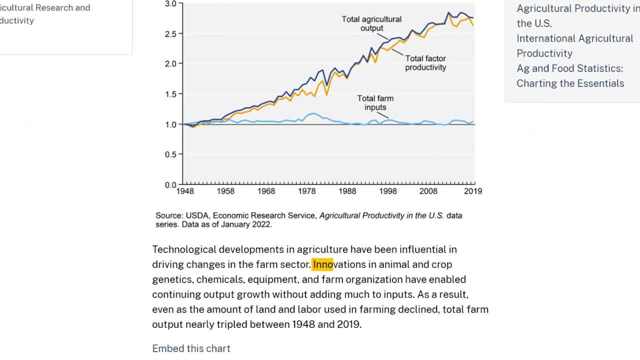 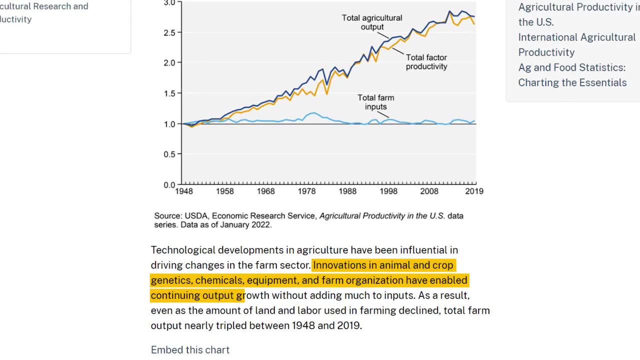 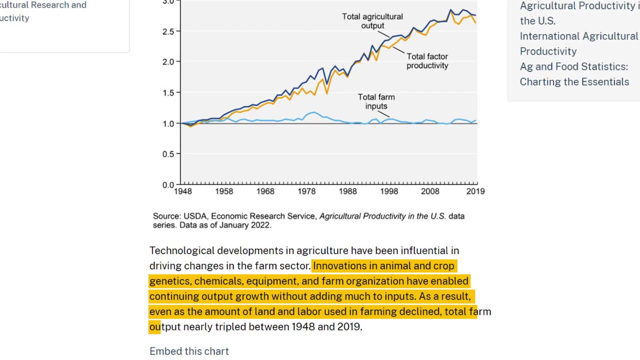 The Department of Agriculture states that this is due to innovations in animal and crop genetics, chemicals, equipment and farm organization, which have enabled continuing output growth without adding much to input As a result, even as the amount of land and labor used in farming declined. 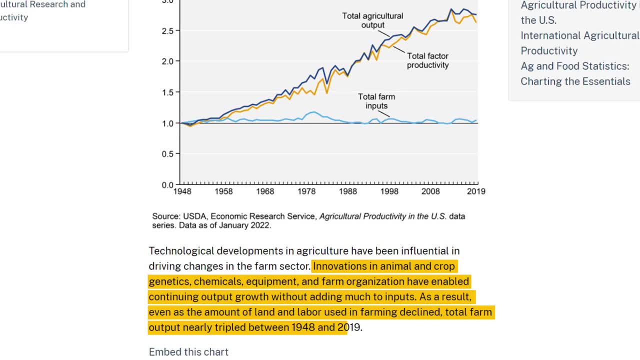 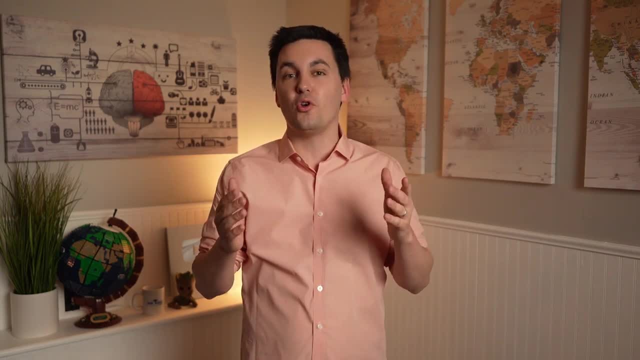 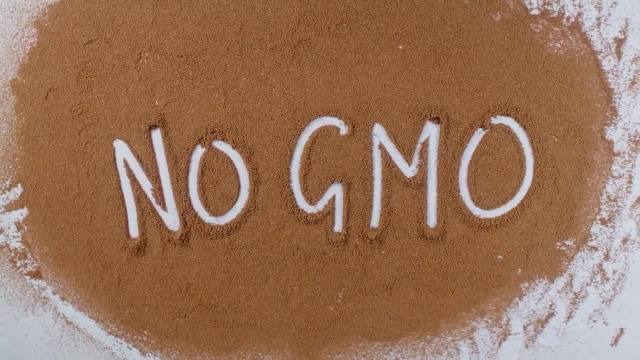 total farm output nearly tripled between 1948 and 2019.. So we can see the impact that technology has had on how we produced our food and how our agriculture is organized. These changes in agriculture have led to some recent debates on how we as a society should produce food.